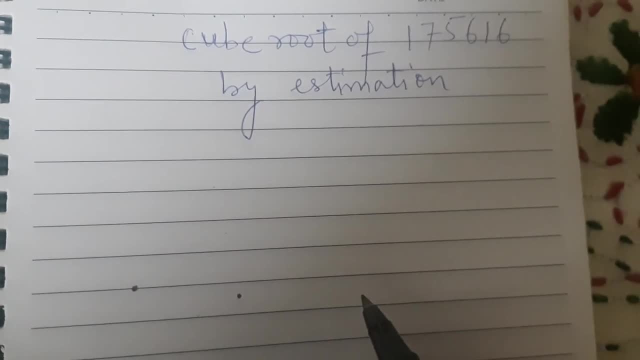 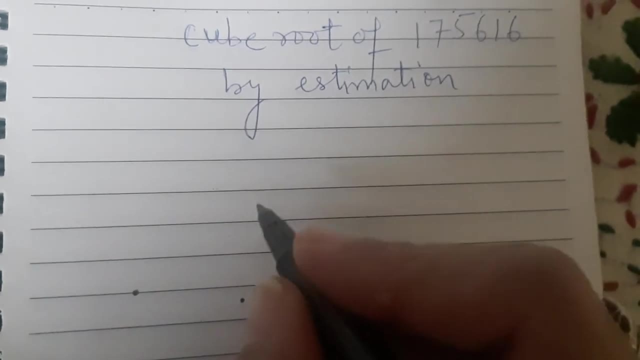 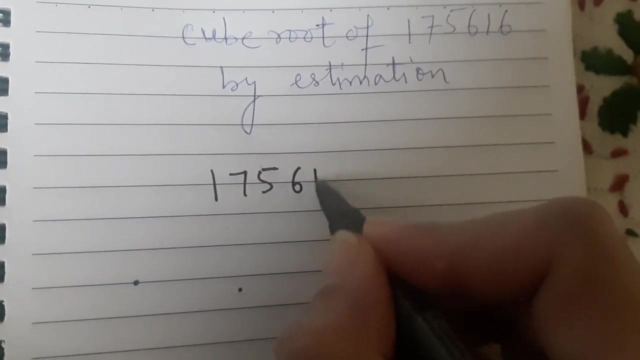 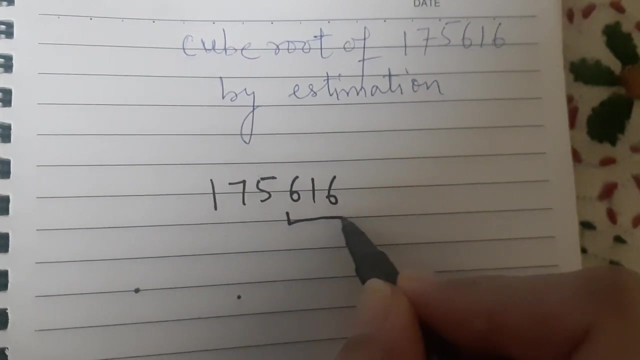 So in the estimation method, what we do is we form the groups of three digits, starting from the right most digits. So let me first write down the number which is given to us: 1,75,616.. So I will be starting from the right most digit and will be making groups of three digits. 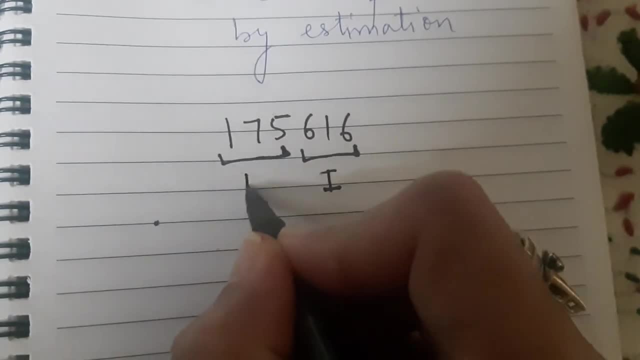 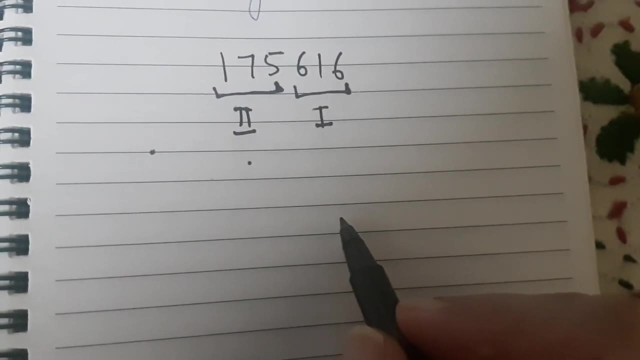 So I will be making groups of three digits. So this is our first group and this is our second group. Now the second step is we have to consider the first group and we have to observe the units digit. What is the units digit of 616?? 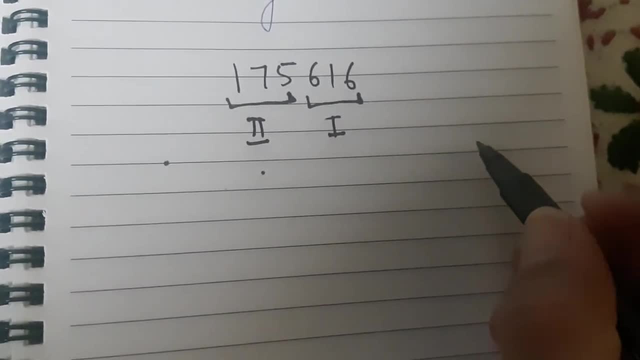 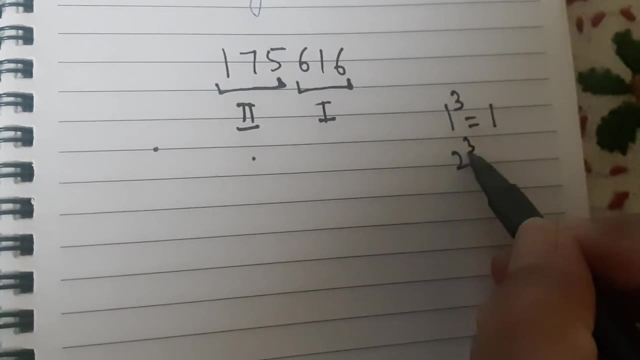 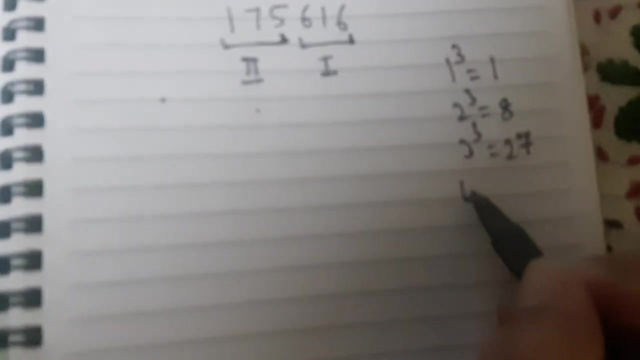 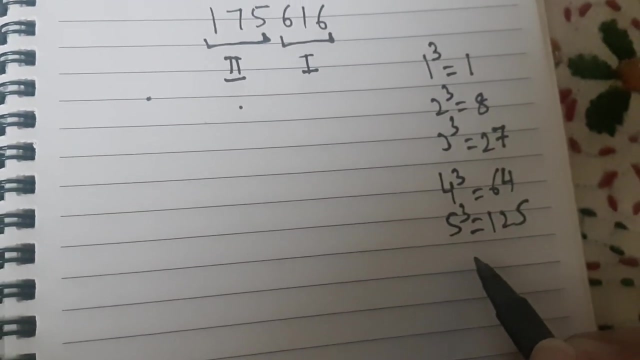 The units digit is 6.. So in your mind just remember cubes of the numbers. So 1 cube is 1,, 2 cube is 8.. 3 cube is 27, then 4 cube is 64, then 5 cube is 125 and 6 cube is 216. 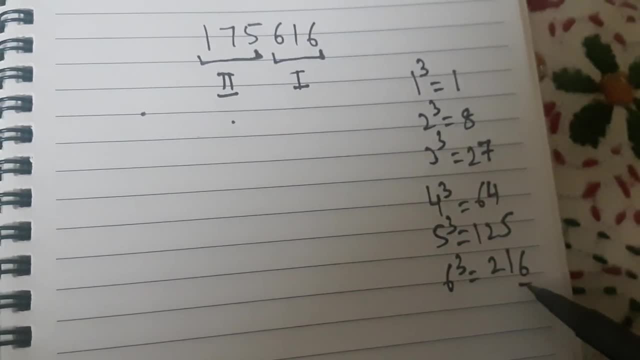 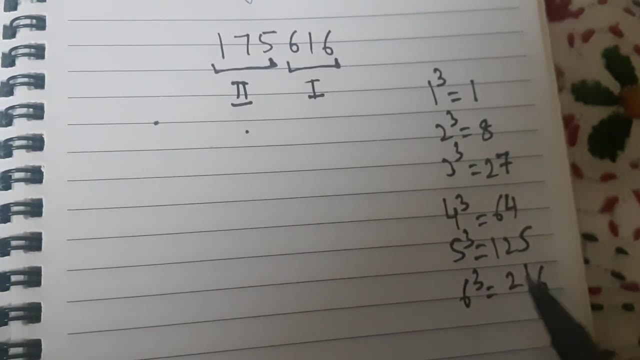 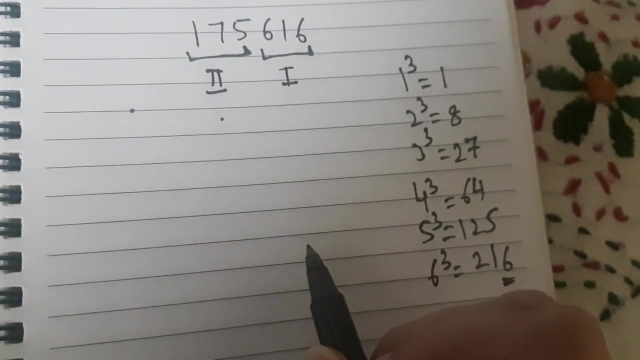 Now observe the unit digit. here I am getting 6 as the unit digit in 6 cube. So this is a clear indication That the unit digit of the cube root of the given number will be 6.. So now we have found the unit digit of the cube root of the given number. 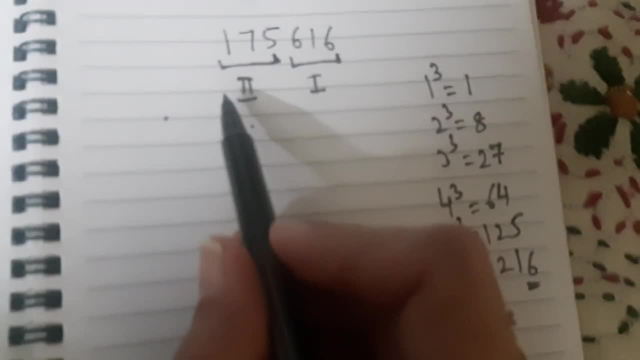 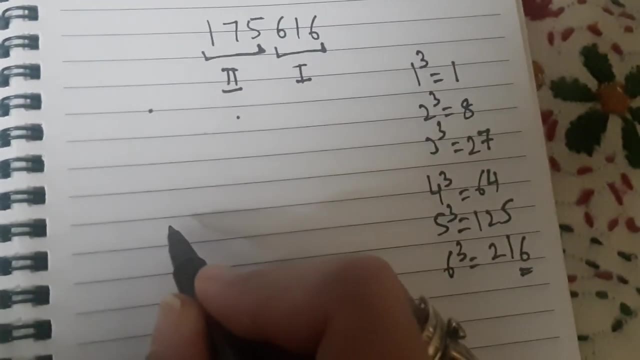 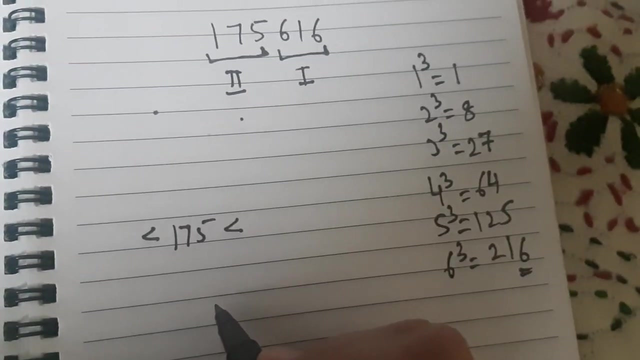 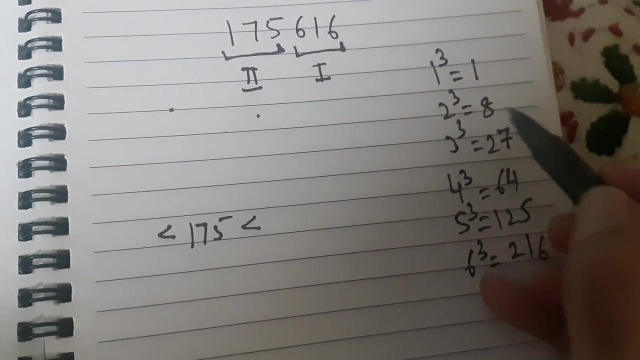 Now what we are going to do is we will be considering the second group. So second group is 175.. Now what you have to see is you have to see two numbers. This is basically the cube Between which 175 lies. So here you can quickly see 175 lies between 5 cube and 6 cube. 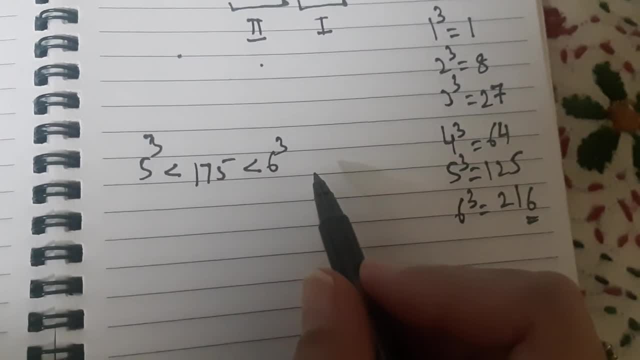 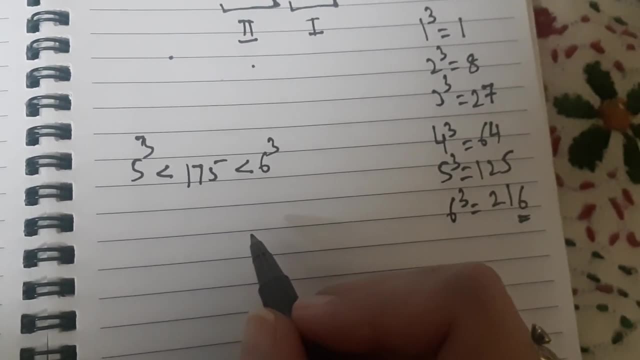 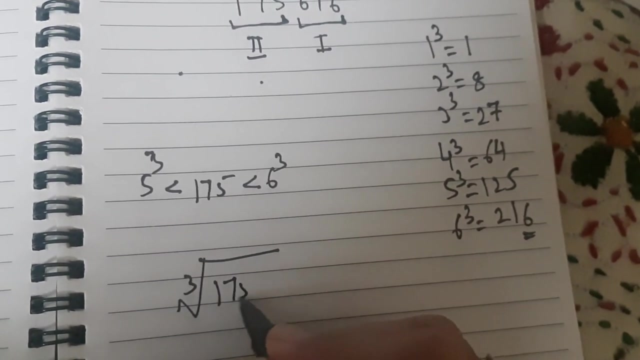 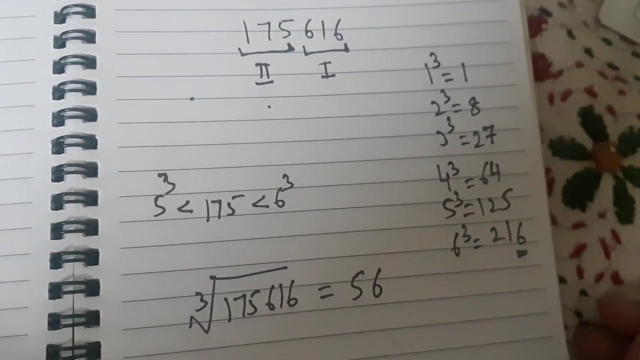 And now you tell me, out of these two, what is the smallest number, 5 or 6.. Yes, you are right, 5 is smaller Number. so the cube root of 1,75,616 will be equal to 56.. So how you are going to write this? 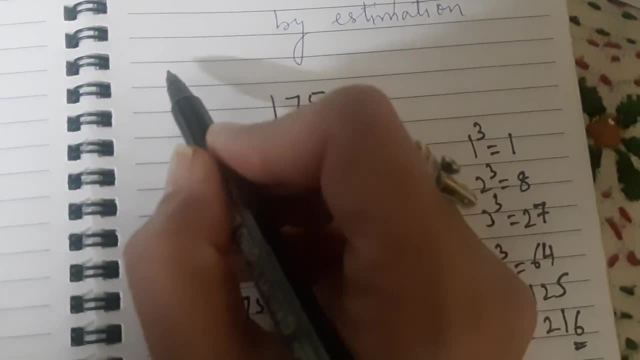 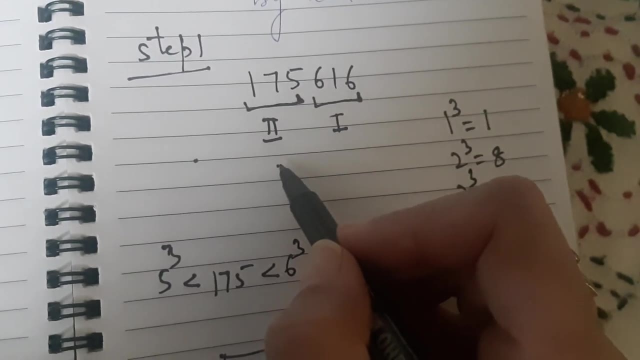 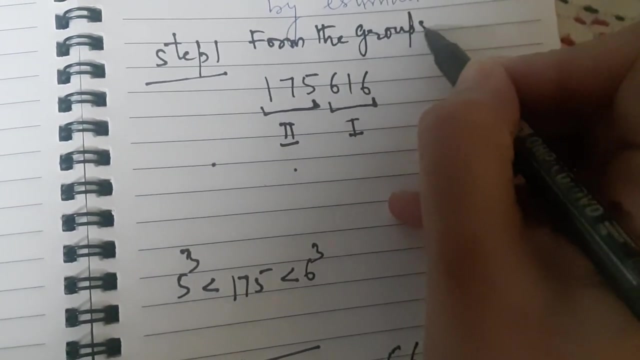 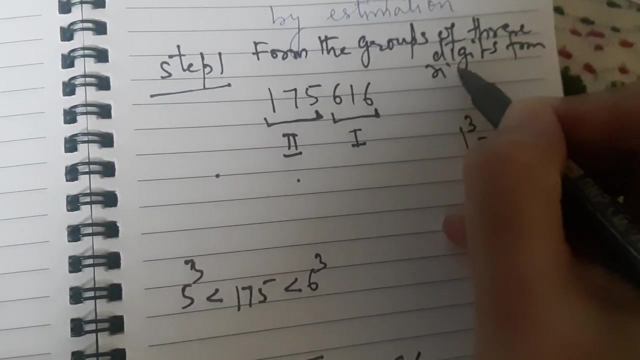 So you will be writing down the steps like here. you will be writing as step 1.. Step 1 is form the groups of three digits starting from the right. So, right here, form The groups of three digits From right. So you have already done here. this is group 1, this is group 2.. 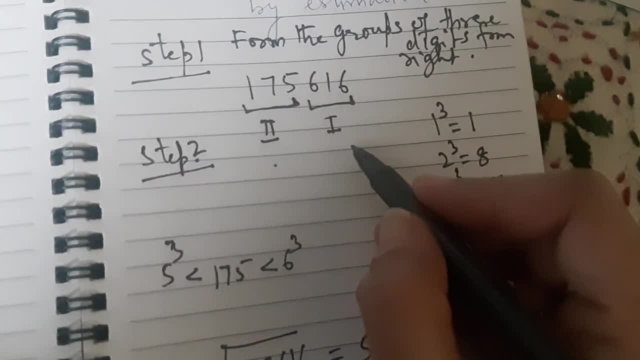 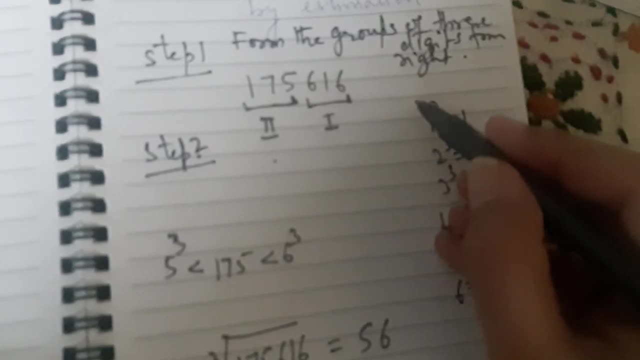 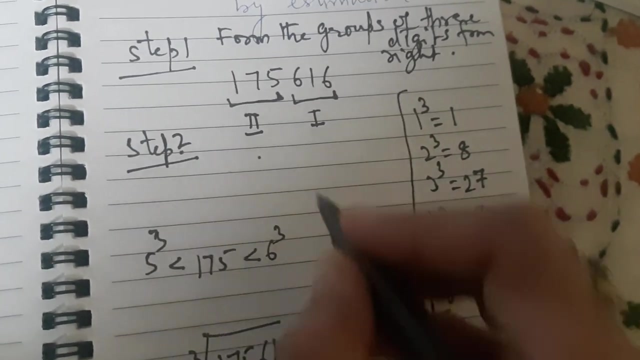 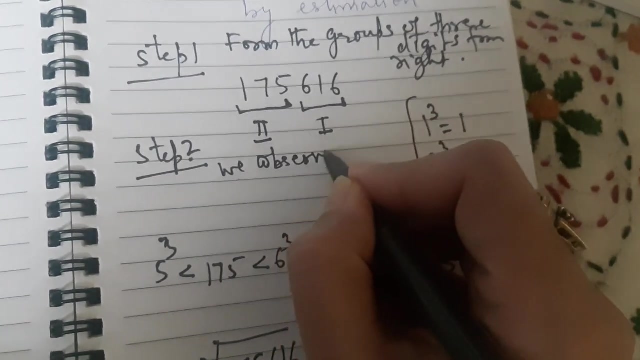 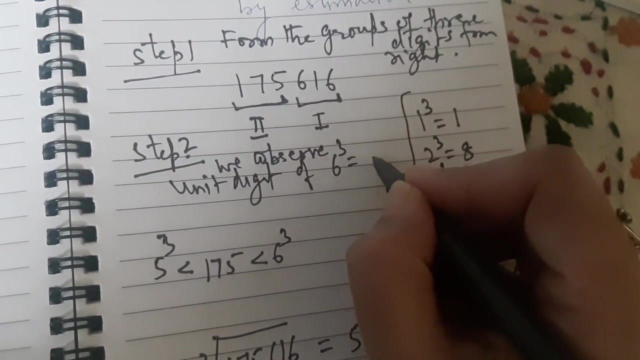 Now what is step 2.. Step 2 is observe the units digit of the first group And you have to see from the cubes Of the numbers where this unit digit is coming up. So we observe unit digit of 6. cube is 6.. 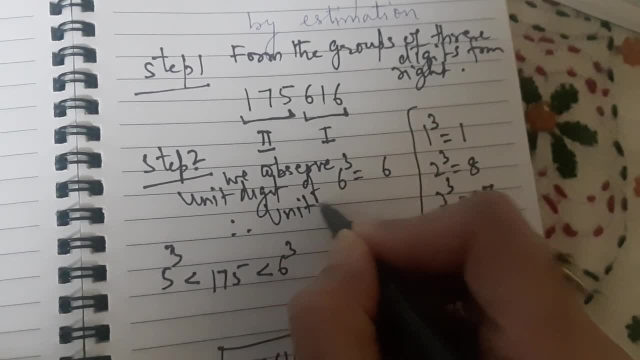 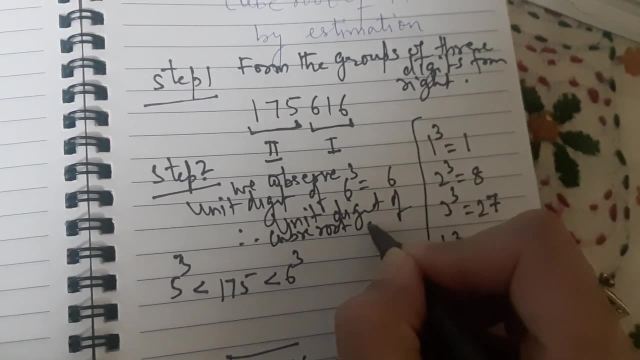 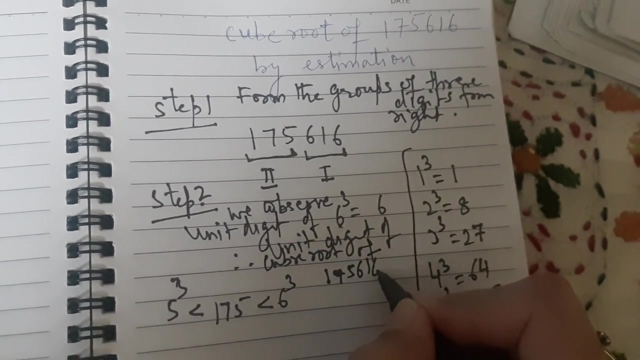 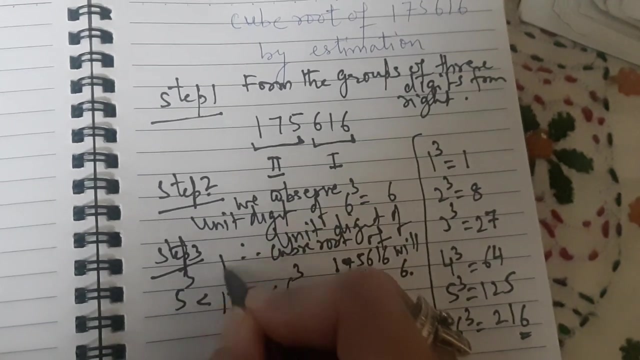 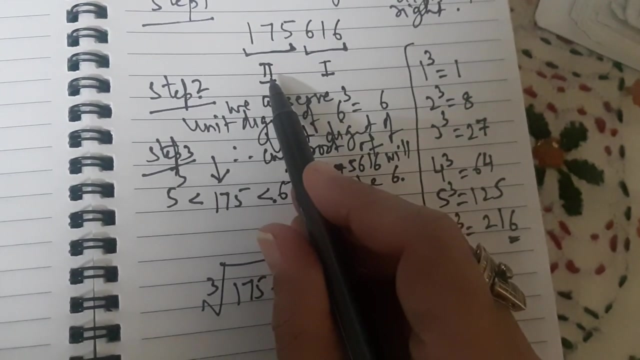 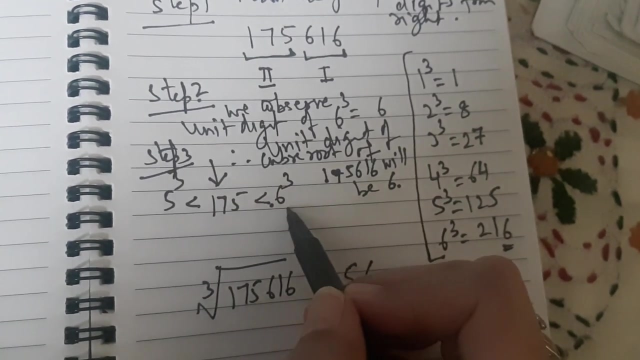 Therefore, unit digit of cube root Of 1,75,616 will be 6.. Now what is step 3.. Step 3 is look for two cubic numbers between which the second group lies. So I have quickly written over here that 5 cube is less than 175 is less than 6 cube. 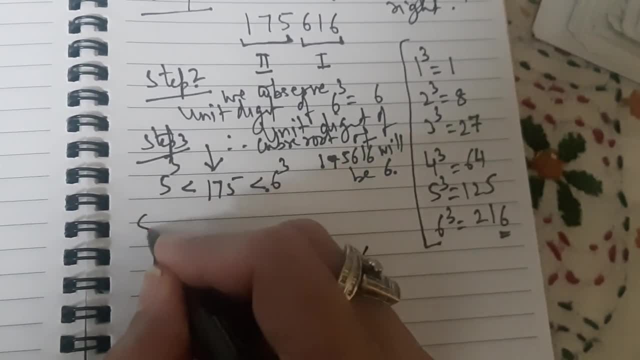 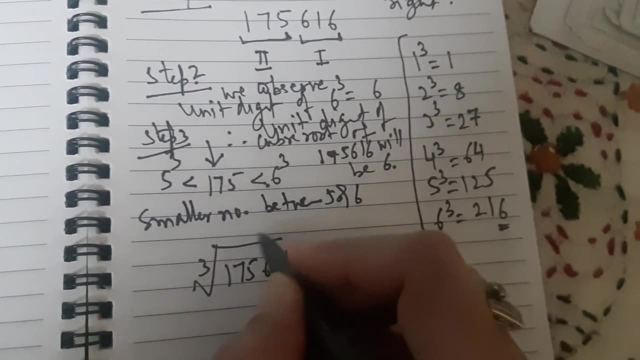 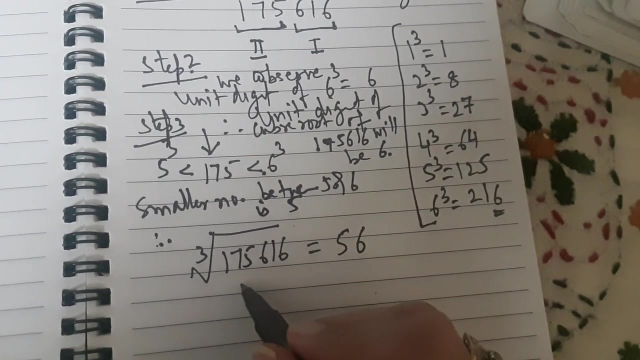 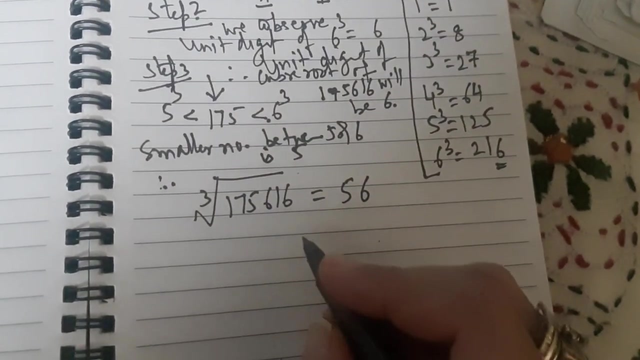 So now you have to see the smaller number. smaller number between 5 and 6 is 5. therefore, cube root of 1,75,616 is equal to 56.. I hope the question is clear to you. So now, using the same method, you now find the: 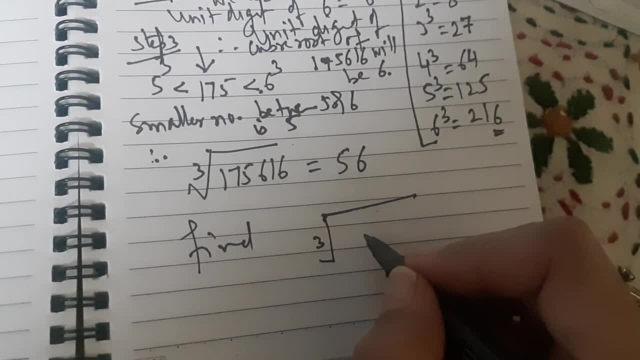 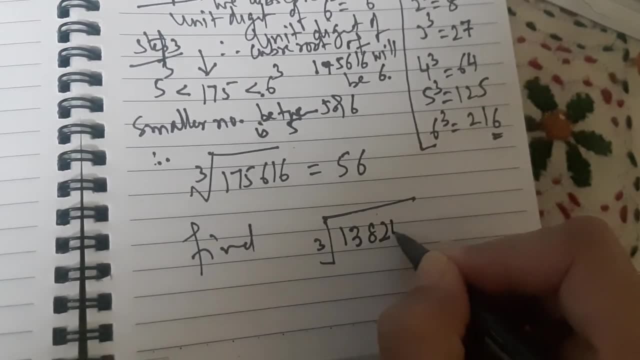 Cube root of. I am giving you one question. okay, 1,3,8,2,4.. Try this.